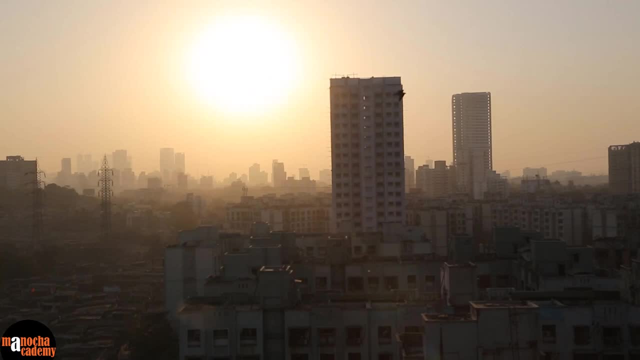 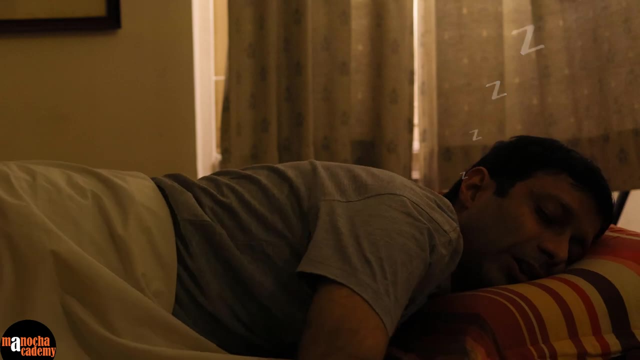 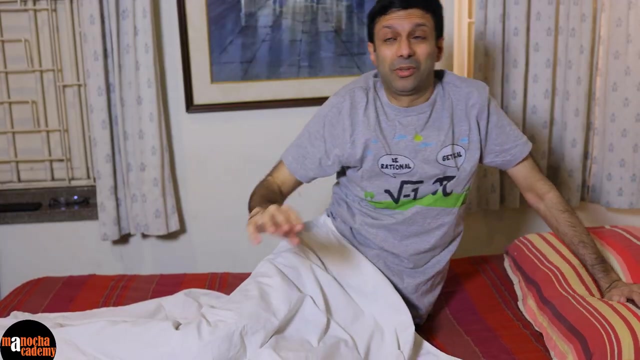 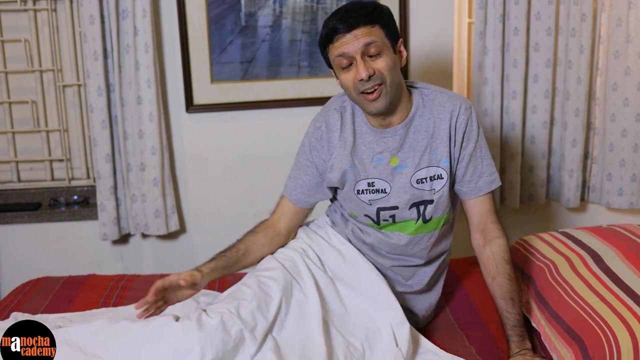 Good morning, Sandeep, Wake up. Huh, Give me five more minutes. Come on, Sandeep, Wake up, You have videos to shoot. Hi friends, I'm sure you felt lazy to get out of bed and start your day right. 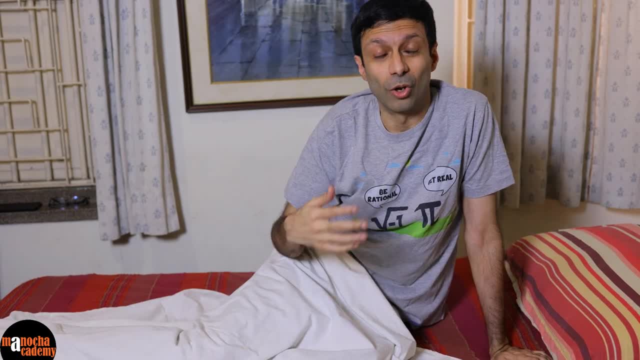 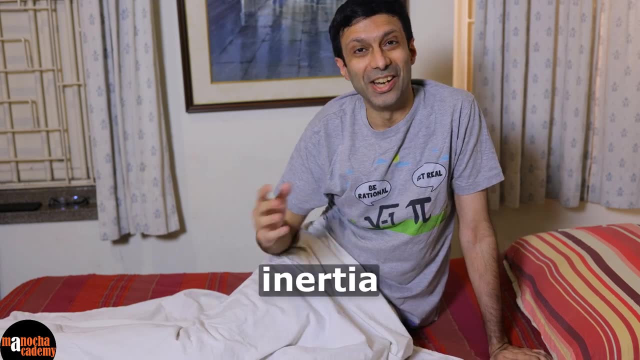 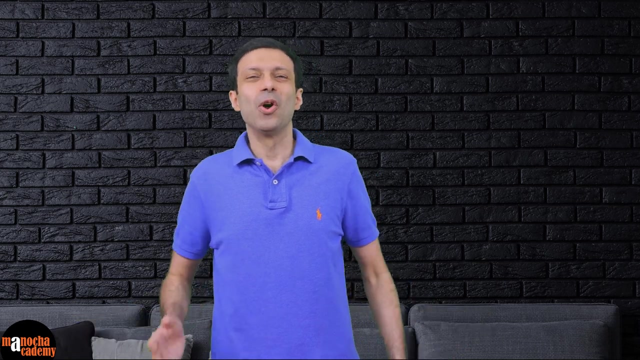 But don't feel guilty about it, Because, according to physics, all bodies feel lazy. In physics, the laziness of a body is called inertia, And that's going to be the topic of this video. Let's understand the concept of inertia with some simple examples. 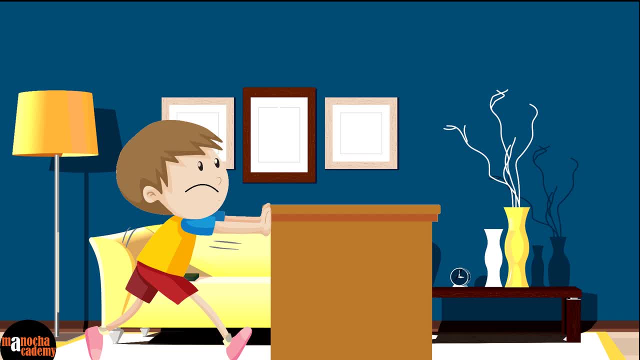 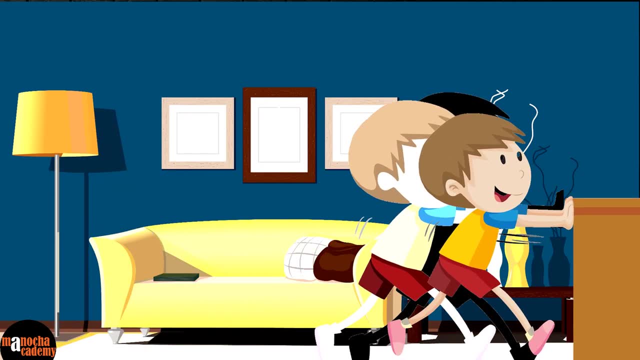 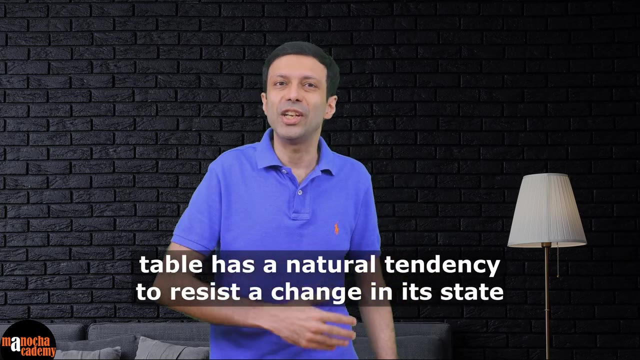 If you try pushing a big table, it's difficult to move it right. We need to apply a very large force to move the table. Why is that? The table has a natural tendency to resist a change in its state. The table is at rest. It's stationary, So it wants to remain at rest. 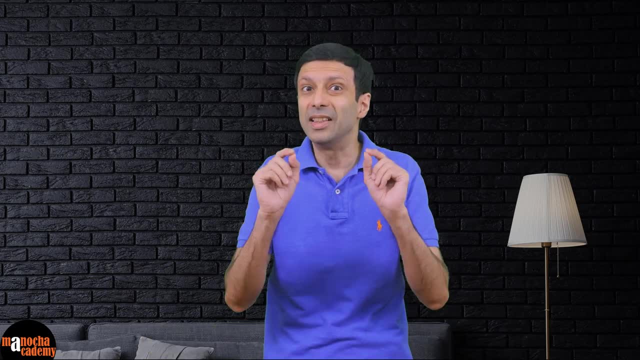 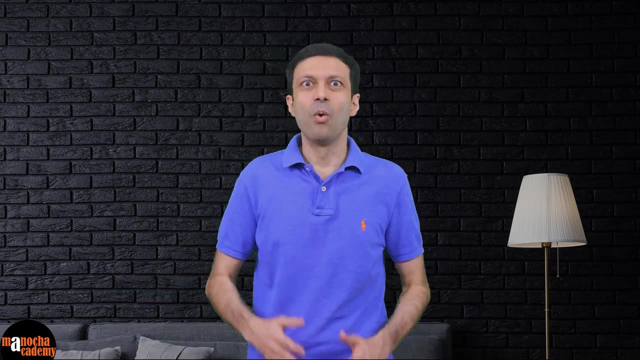 It's lazy, It doesn't want to move. This is called inertia of rest. Now, if you consider the example of a moving body, If you have a moving ball, what do you need to do to stop it? You need to apply a force. 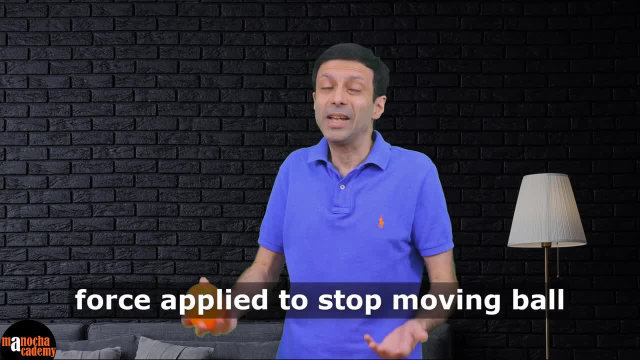 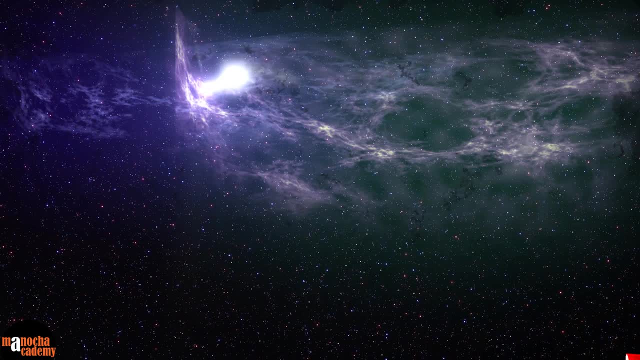 As you saw here, I applied a force to stop the moving ball, Otherwise it will keep on moving right. Obviously we are ignoring the air friction here. Another example is a rocket in space that wants to keep on moving. It does not want to stop. 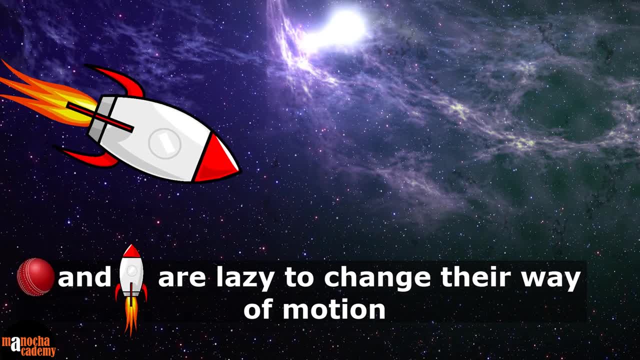 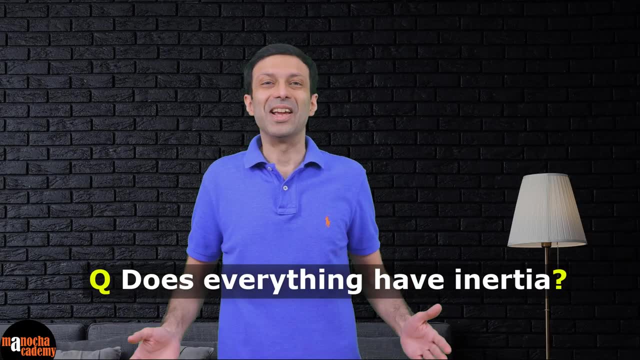 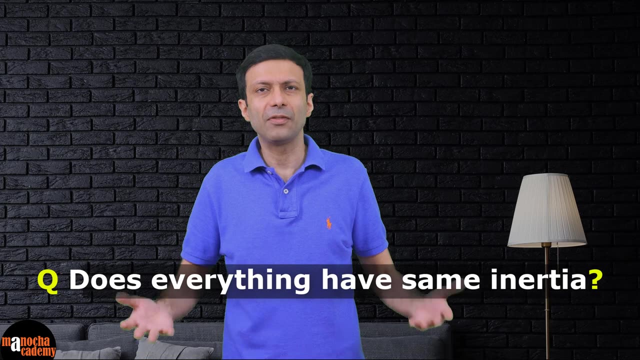 The ball and the rocket. they are lazy to change their state of motion. This is inertia of motion. Does everything have inertia? The answer is yes. So basically, everything is lazy. Now, do all the bodies have the same inertia? What do you think? 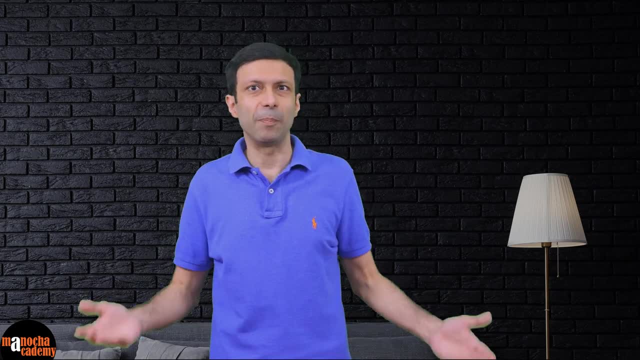 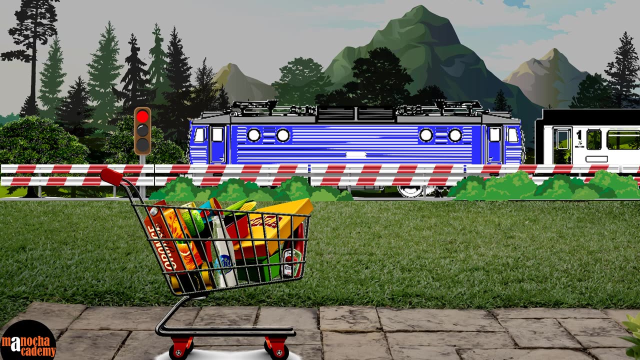 The answer is no. So what does inertia depend on? Let's find out. Consider the example of a shopping cart and a train. Let's say both are at rest. Which one do you think has more inertia? Think which one will be more difficult to move. 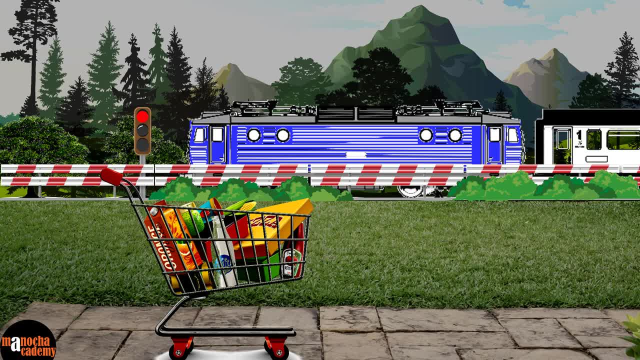 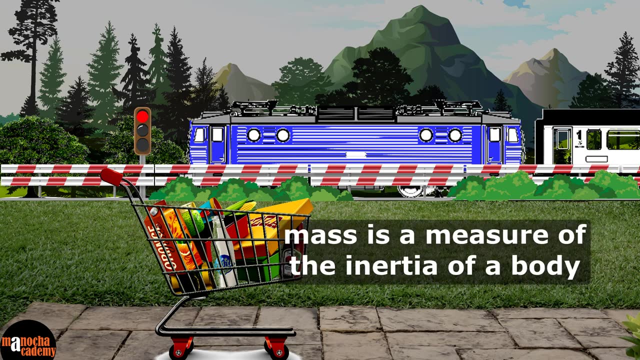 Obviously, it is more difficult to move the train as compared to the shopping cart, As the train is much more heavier than the shopping cart. So inertia depends on the mass of the body. Greater the mass, greater will be the inertia. In fact we say that mass is a measure of the inertia of a body. 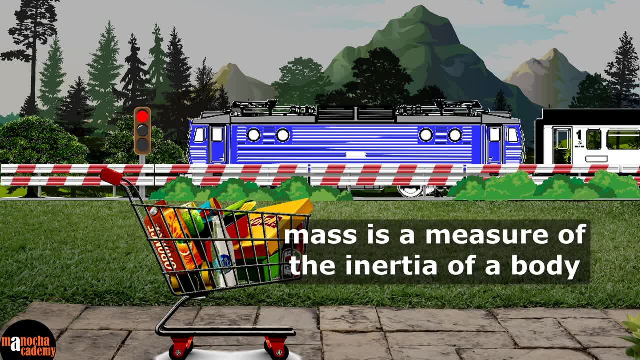 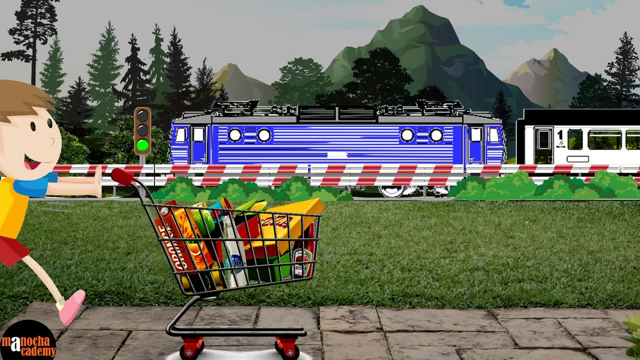 And the same also applies if both the shopping cart and the train are moving. Let's say, they are moving at the same speed. Which one do you think is more difficult to stop, The shopping cart or the train? Again, the answer is the train, right. 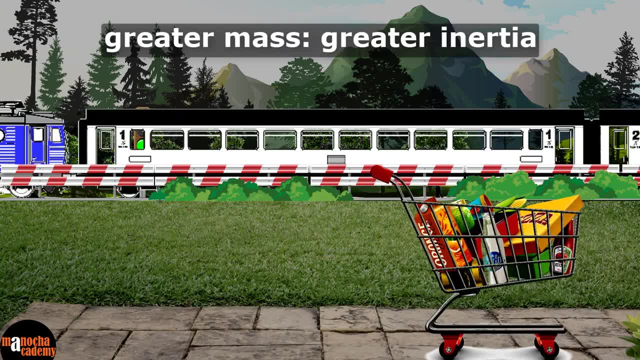 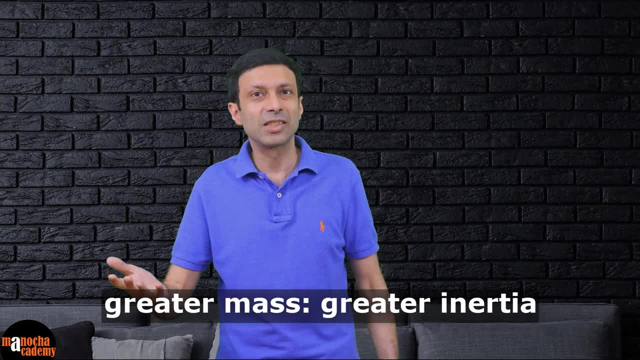 You don't want to be standing in front of a moving train because it has greater mass, So it has greater inertia of motion. So remember, greater the mass, greater will be the inertia, Whether you talk about inertia of rest or inertia of motion. 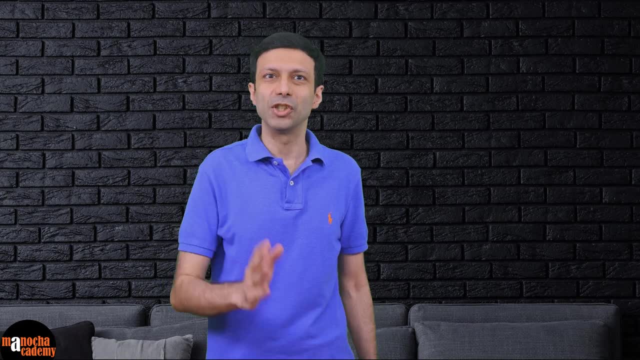 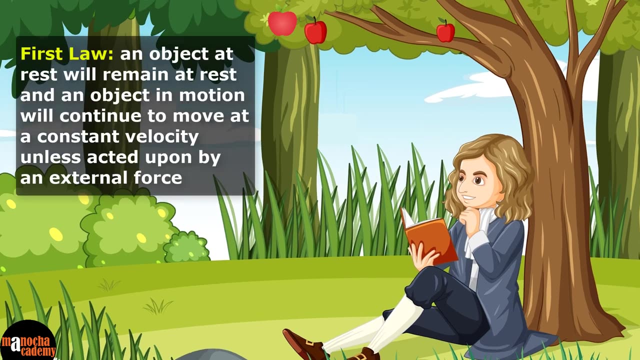 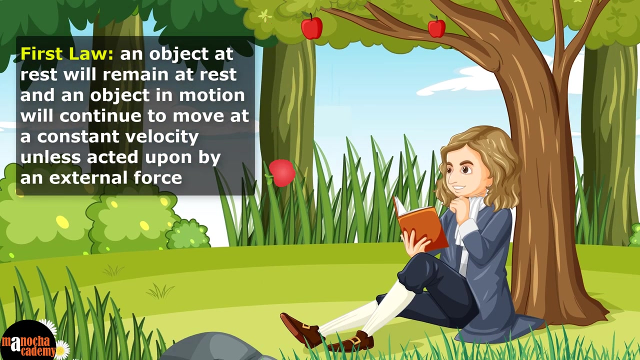 Sir Isaac Newton first described the concept of inertia in his famous laws of motion. In his first law of motion he stated that an object at rest will remain at rest And an object in motion will continue to move at a constant velocity unless acted upon by an external force. 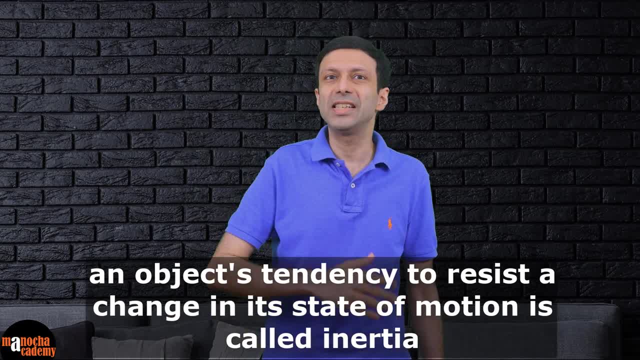 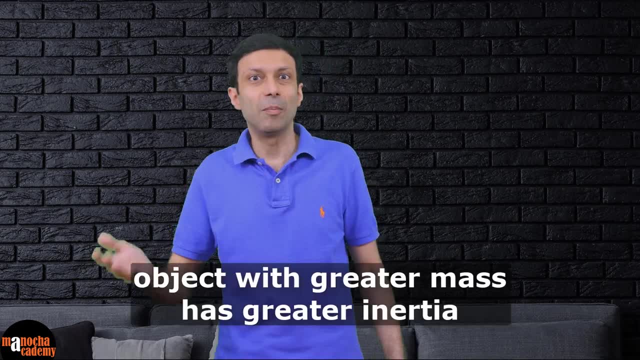 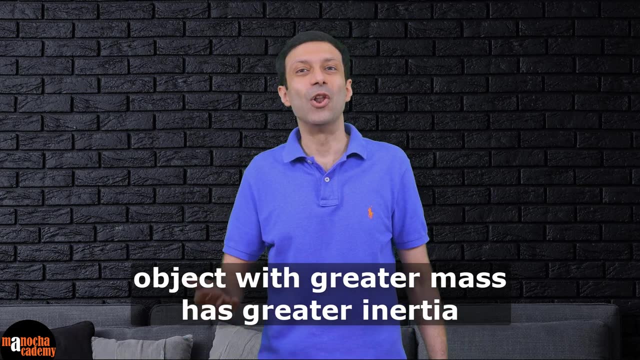 In other words, an object's tendency to resist a change in its state of motion is called inertia. And remember, as we discussed, greater the mass of the object, greater will be its inertia. That is why the first law is also known as the law of inertia. 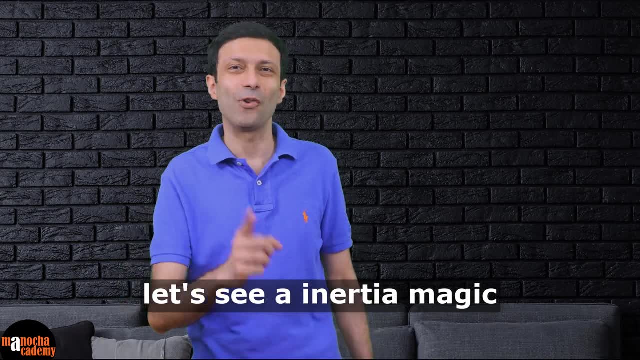 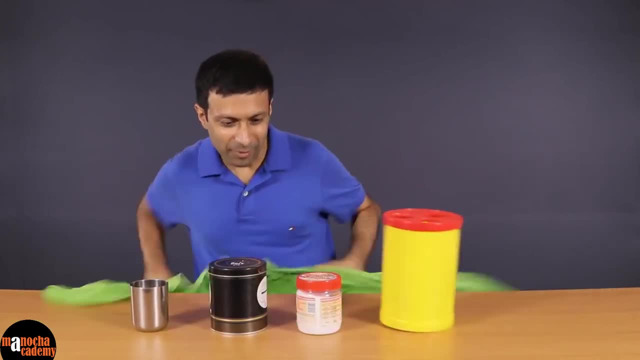 Are you ready to see a tablecloth magic that's based on this law of inertia? Here it is Ready: One, two, three. Did you like it? Did you like the magic trick? Luckily, I didn't drop any of the objects on the table. 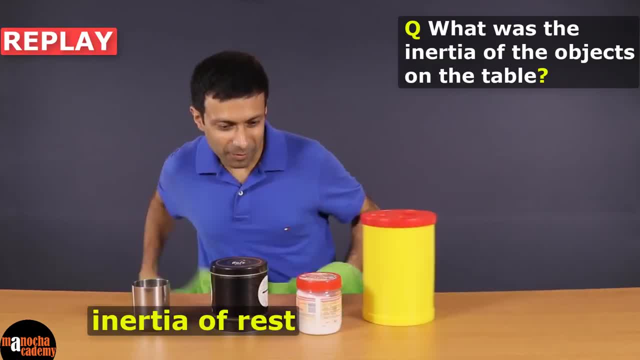 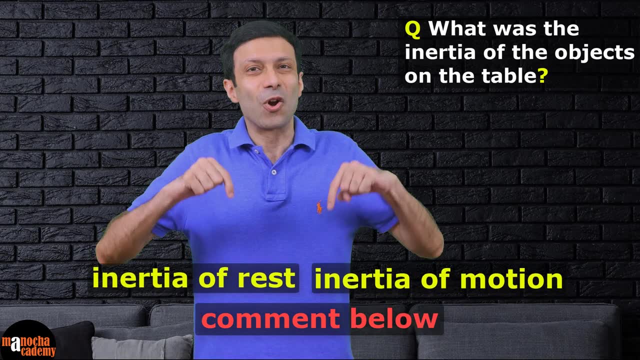 Now, can you tell me the objects on the table? were they in the inertia of rest or inertia of motion? What do you think? Do let me know your answers by putting it in the comments below. I'm looking forward to reading your answers.